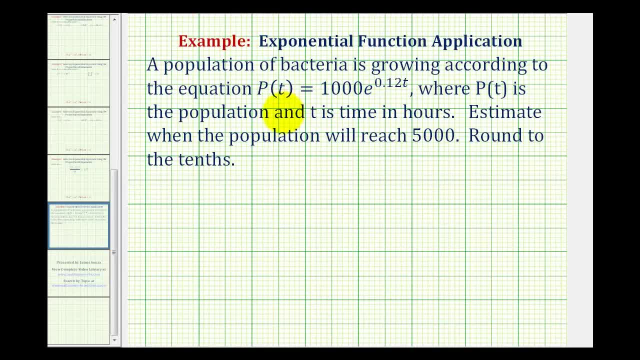 A population of bacteria is growing. according to the equation, p of t equals 1,000 times e, raised to the power of 0.12t, where p of t is the population and t is the time in hours. We want to estimate when the population will reach 5,000 and round our answer to the nearest tenths. 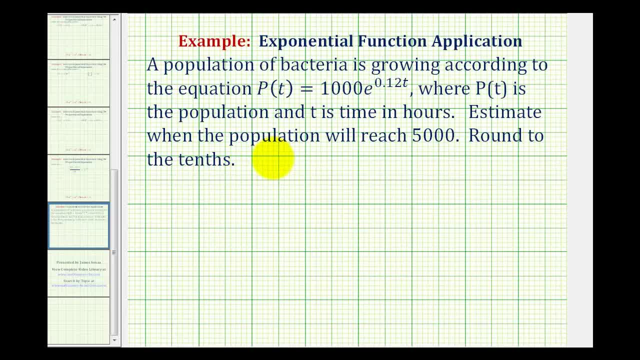 We will be solving this type of problem using logarithms very soon, but for right now we're going to solve this problem using the graphing calculator. We'll use the table feature as well as the graphing feature to solve this problem. So we're given this equation here that tells us the population of the bacteria at t hours. 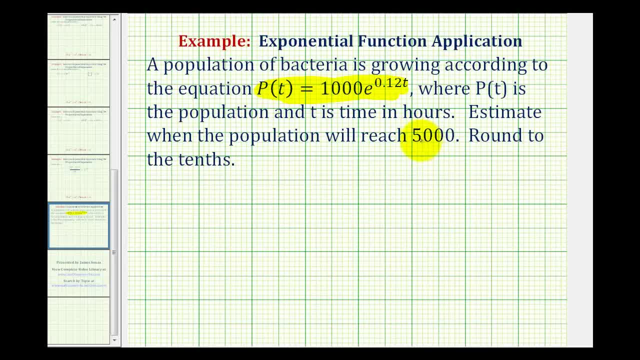 And we want to know when the population, or p of t, reaches 5,000.. So we're trying to solve the equation: 5,000 equals 1,000 times e raised to the power of 0.12t. Let's start by entering the function into our graphing calculator. 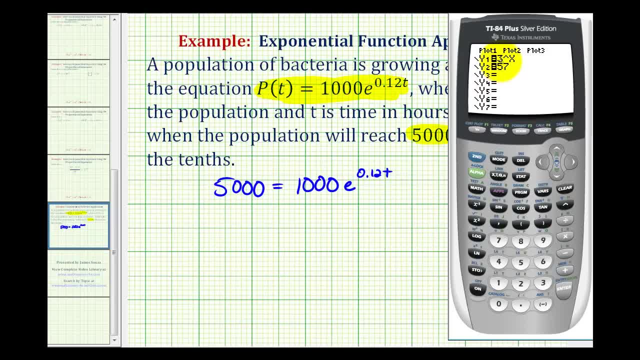 So we're going to press y equals clear out any old functions. So we'll just press clear, clear, go back up to y1 and type in the population function, So we'll have 1,000. and then for e, we press second ln. 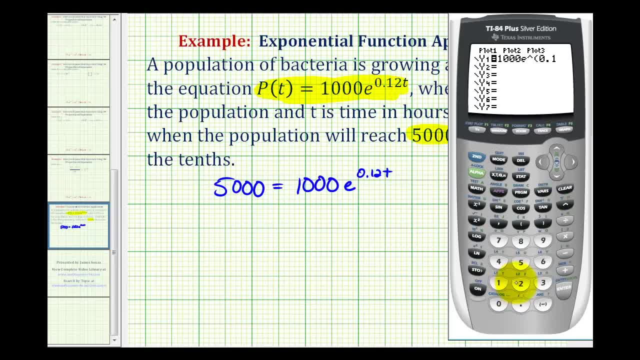 Our exponent is 0.12 times t, which we'll just use x. And now let's go to our table set by pressing second window. Let's go ahead and start the table at 0 and increase the values by 1.. So now, if we go to our table by pressing second graph, we can get an idea of when the population will reach 5,000.. 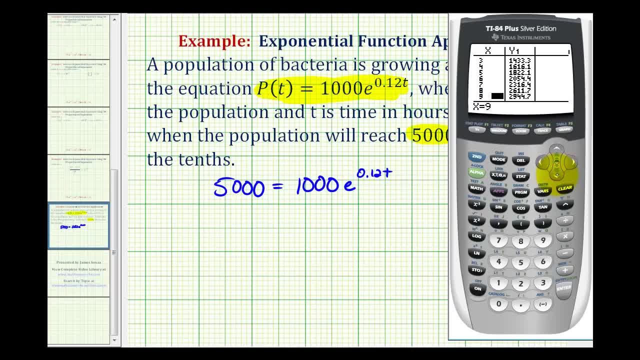 So if we scroll down, notice how it's somewhere between 13 and 14 hours, To be more precise, we could go back to the table set And start the table at 13 this time and make the change in table tenths So 0.1 and narrow down our estimate to the tenths.